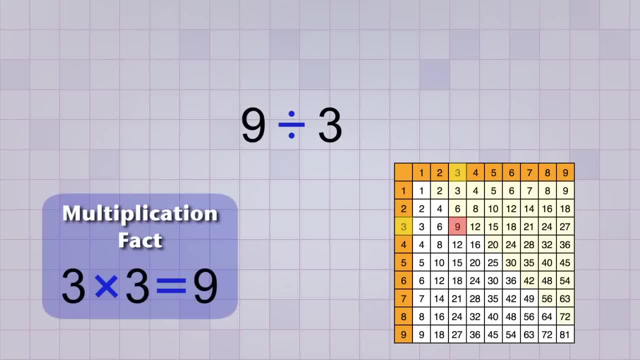 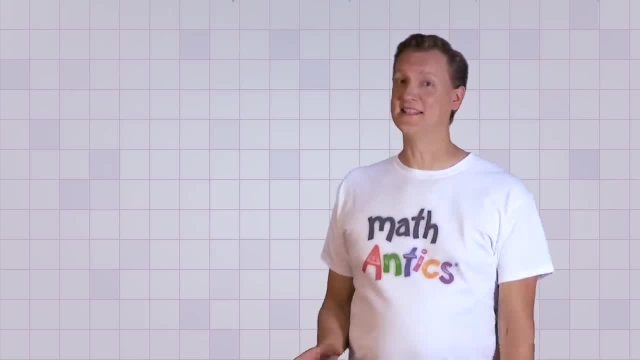 or that it's an answer on the multiplication table. then you can see that since 3 times 3 is 9, then 9 divided by 3 is 3.. It's that simple. Well, at least it WAS that simple when you learned about the fact families. 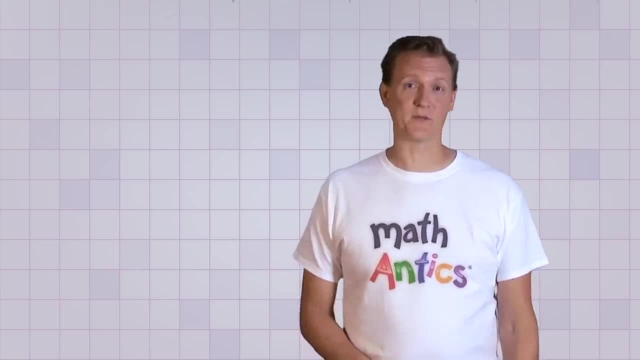 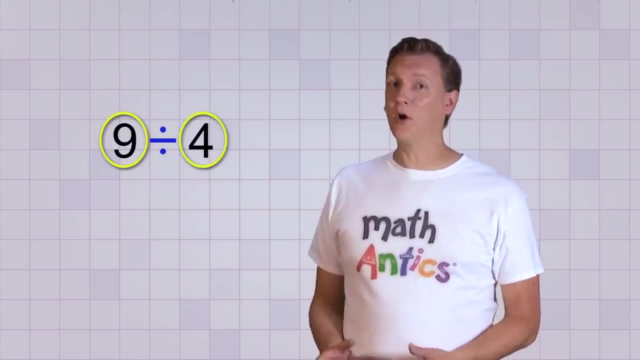 Now it's going to get a little bit tricky because most division problems aren't quite this easy, Like this one: 9 divided by 4.. The trouble here is that 9 and 4 aren't part of a fact family, So you can't just find the answer on the multiplication table. 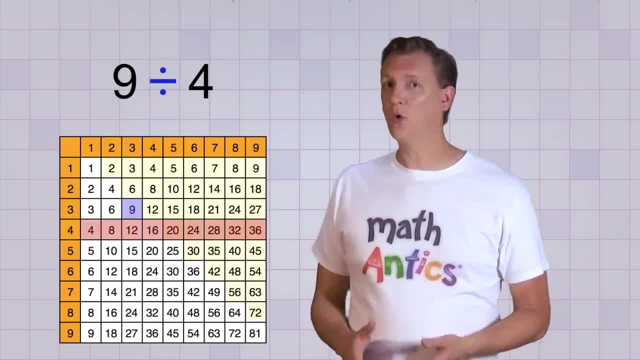 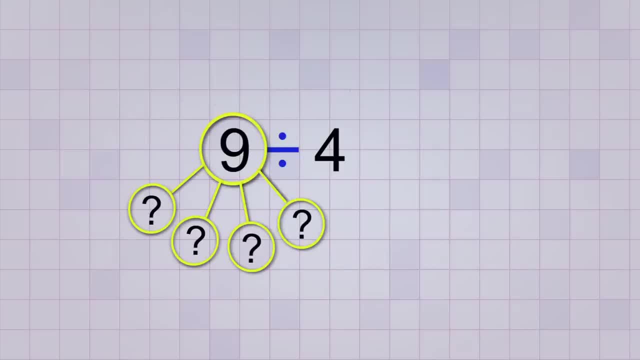 That's because 9 is not a multiple of 4.. There's no whole number that you can multiply 4 by and end up with 9.. That means that 9 can't be divided equally into 4 groups without having something left over. 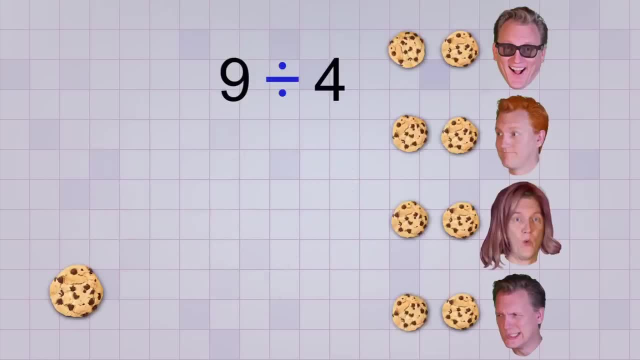 Like if you had 9 cookies and 4 kids, each kid could have 2 cookies but there would be 1 left over And in division that leftover amount is called the remainder. So the answer to 9 divided by 4 is 2 with a remainder of 1.. 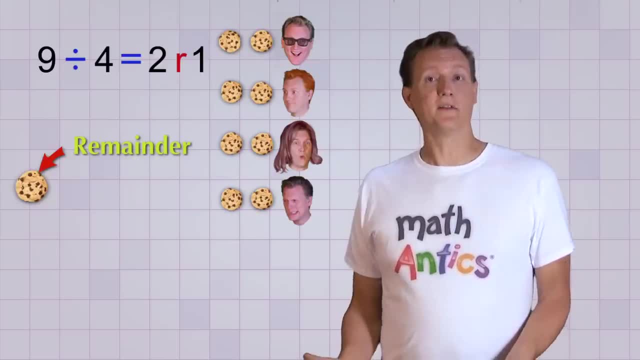 So the answer to 9 divided by 4 is 2 with a remainder of 1.. So the answer to 9 divided by 4 is 2 with a remainder of 1.. Alright, so it's not that hard to figure out a simple division problem when you have a picture like this. 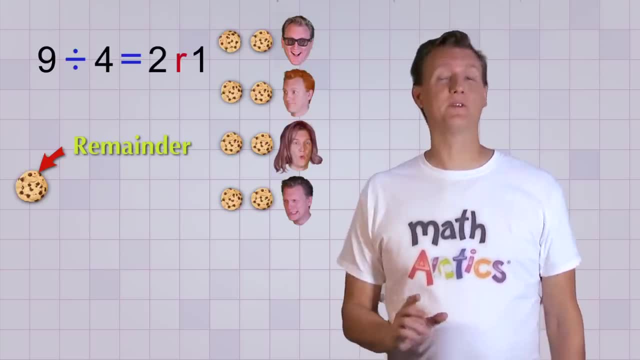 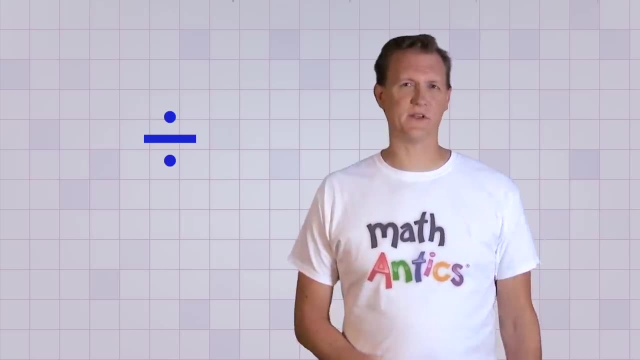 But what about when we just have numbers? To do that, we use a special division procedure. Up until now you probably have used this division symbol the most. It works well for very simple division problems like the ones in our fact families. 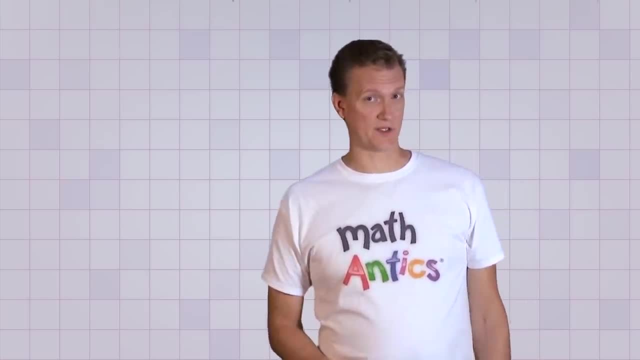 But now that we're going to be doing some harder problems, we need a new division symbol. This one, This division symbol, is special because it's almost like a stage that will help us figure out how to divide a number, Because it's almost like a stage that will help us figure out how to divide a number. 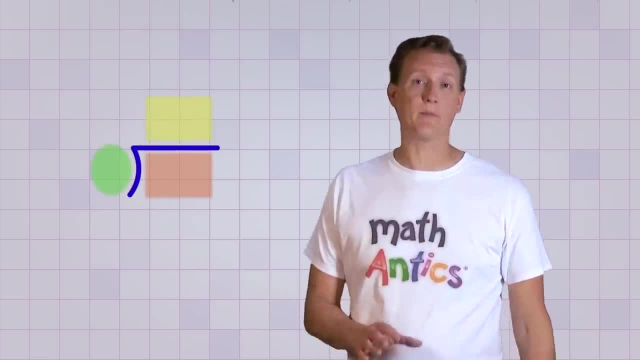 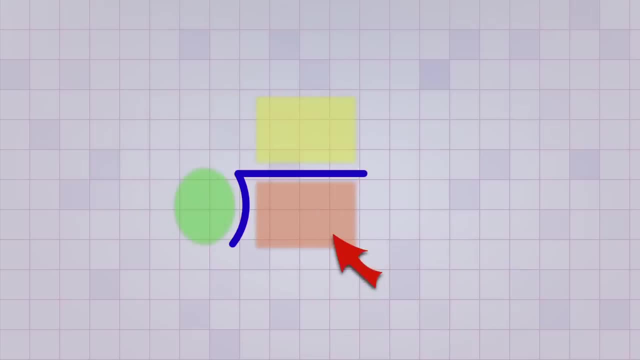 So we'll use this division symbol to solve our division problem And there's three special areas of this stage where the three main parts or characters of our division problem will go. The first area is here, under the long horizontal line on our division symbol. 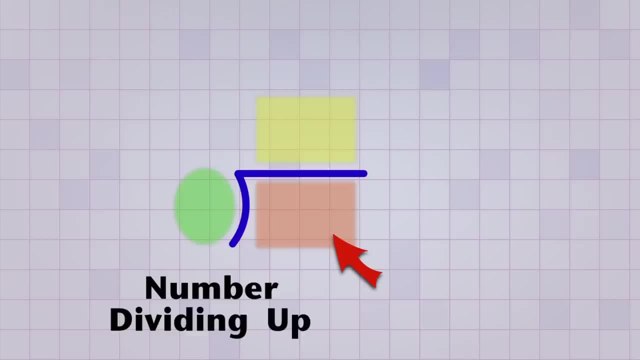 This is the area where we put the number that we'll be dividing up. The fancy math term for this is the dividend. Most of the time, the biggest number will go here, because we usually start with a big amount and want to divide it into smaller groups. 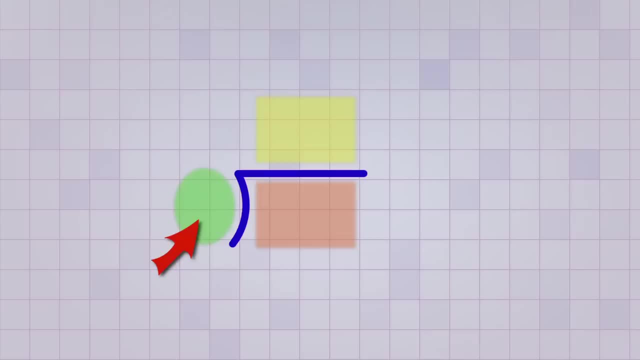 The second area is out in front of the curved part of the division symbol. This is the area where we put the number we'll be dividing by The math term, for that is the divisor. In other words, this number will tell us how many groups we'll be dividing our big amount into. 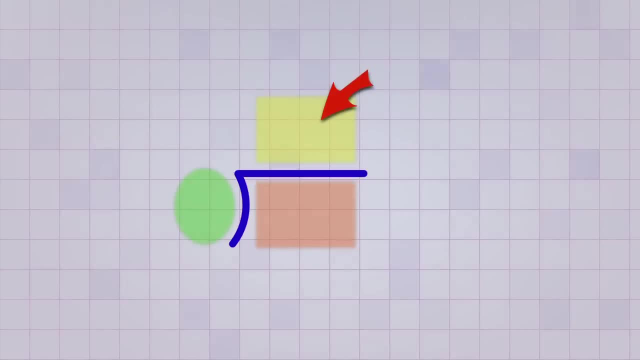 And the third area is up above the horizontal one. This is where our answer will go, once we figure out what the answer is. The answer to a division problem is called the quotient. The answer tells us how many we'll end up with in each group. 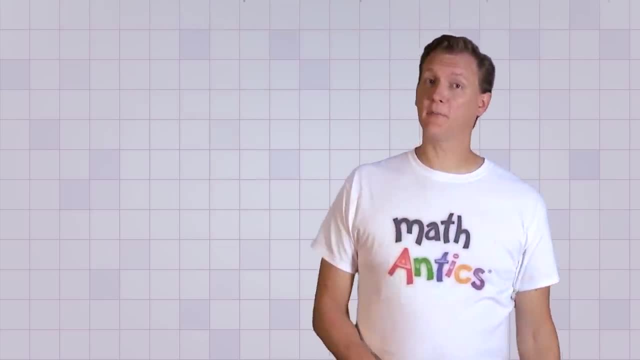 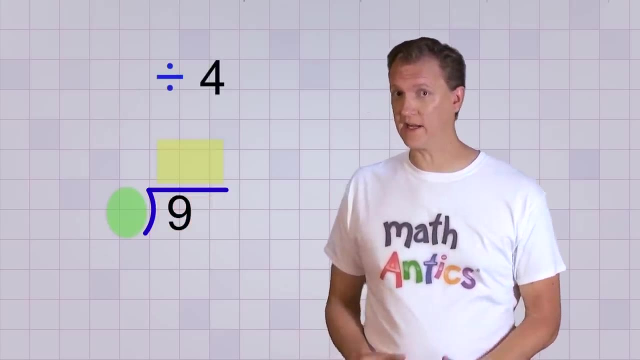 So whenever you have a complicated division problem to do, the first step is to rewrite your problem in this form. If you have 9 divided by 4 like this, you put the 9 down here. that's the number we're dividing up. 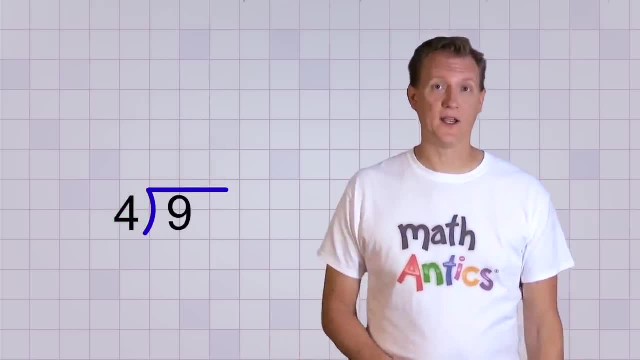 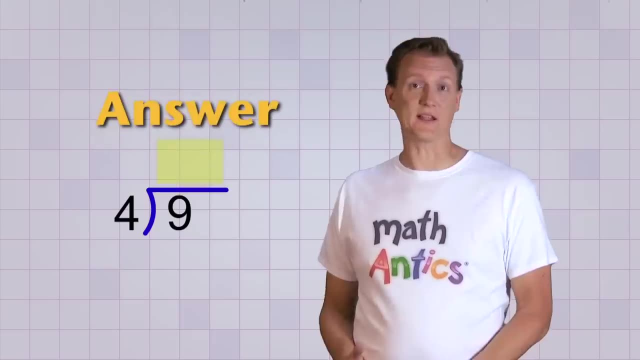 and you put the 4 out here. that's the number we're dividing by, And you're ready to start the next step of the procedure. The next step is the most important step, because it's where you figure out the answer. And to figure out the answer, which is how many you'll end up with in each group after you divide. 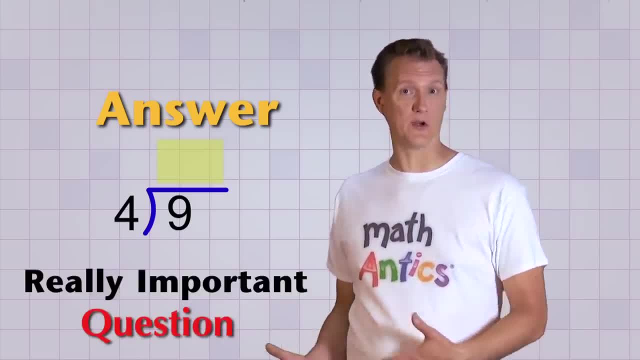 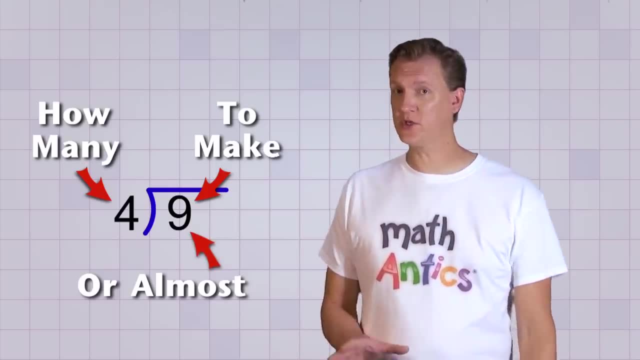 you have to ask yourself a really important question involving the other two numbers. The question is: how many 4's will it take to make 9, or almost 9?? And the key to answering this question is for the number to be just right. 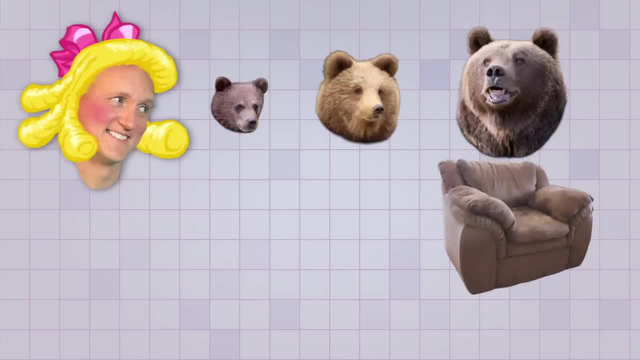 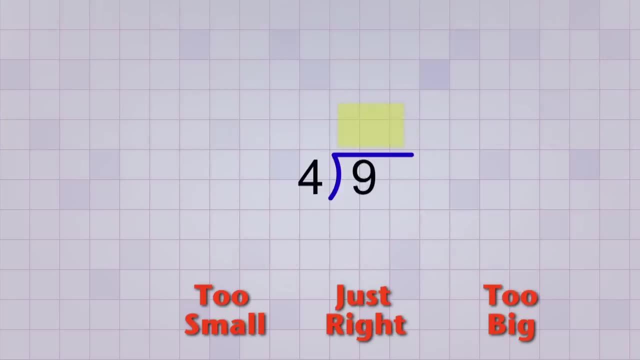 Do you remember the story of Goldilocks and the Three Bears, How one chair was too big and one chair was too small, but the other chair was just right? Well, it's the same way with our division problem. If I choose an answer that's too big or too small, it'll cause trouble for me. 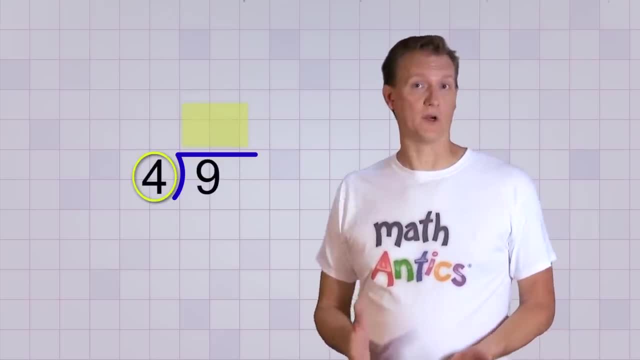 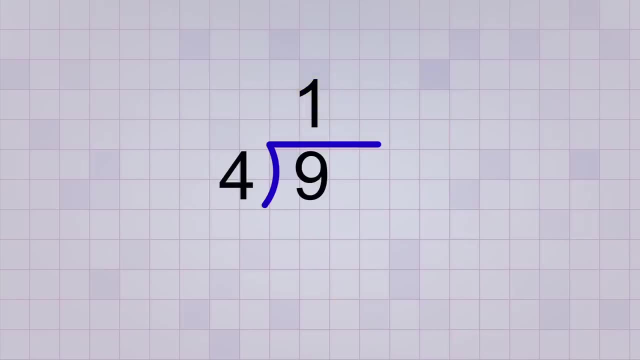 Here's what I mean. Let's say that I decide that I only need one 4 to make 9.. So I'll write a 1 up here in the spot for the answer. Well, now the next step in the procedure is to multiply that answer. I put there the 1,. 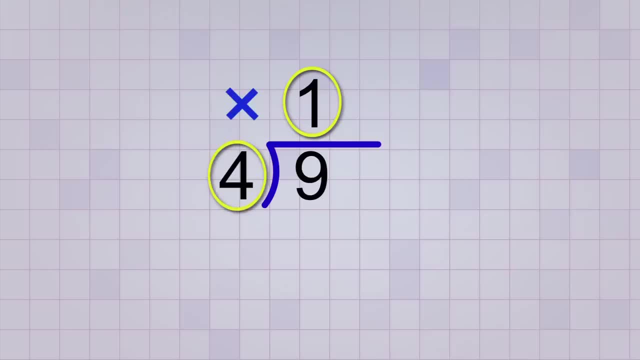 by the number of groups out front here, the 4.. And I write the answer to that multiplication down below the number I'm dividing up, the 9.. I do that so I can subtract that amount from the 9 to see how much I'm going to have left over. 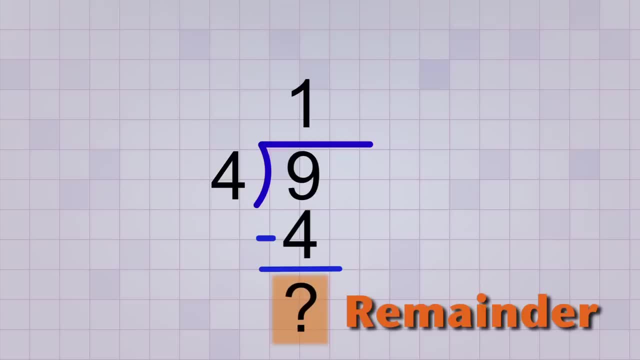 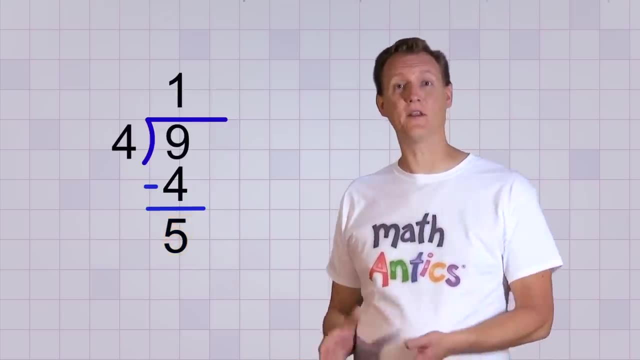 to see how big the remainder will be, And when I do that, I see that 9 minus 4 will give me 5. That's a pretty big remainder. In fact, the remainder is bigger than the number I'm dividing by, and that's why this answer is trouble. 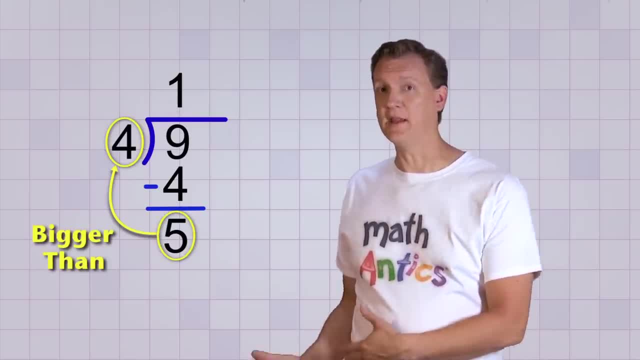 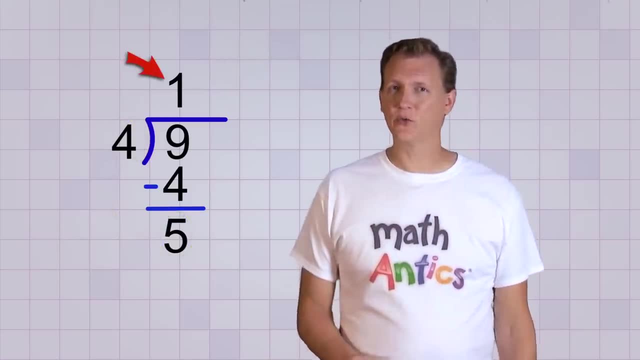 If the remainder is bigger than the number you're dividing by, it means that you should have picked a bigger answer, because each of the groups you're dividing up into could have gotten more than they did. Your answer was too small, and so the remainder was too big. 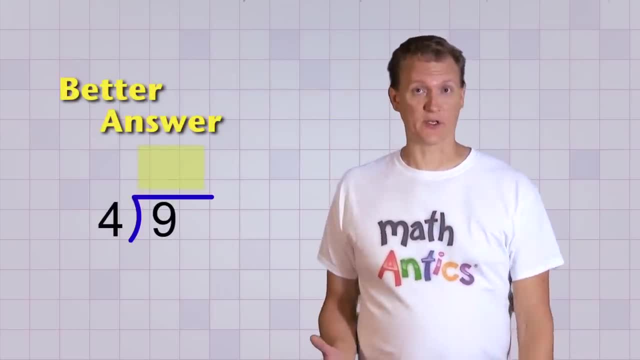 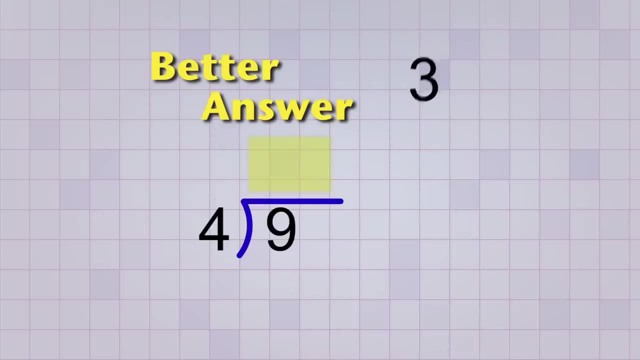 Okay, then I guess I'd better come up with a better answer to the question: how many 4's will it take to make 9, or almost 9.? This time I think I'll pick 3.. So I put a 3 in the answer space and then I follow the next step of the procedure, like I did before. 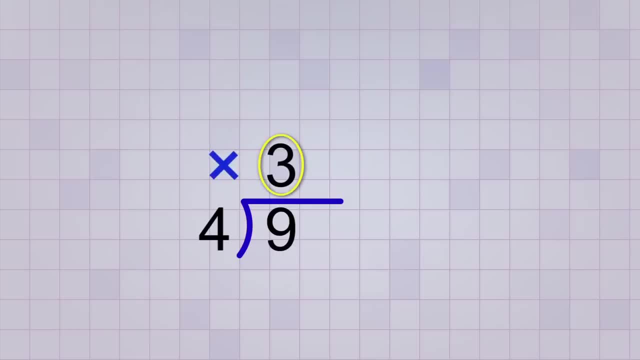 I multiply the answer I chose- 3, by the number of groups, 4, and I write the answer to that multiplication problem: 12, down below the number we're dividing up the 9.. Now I can subtract that number to see what my remainder will be. 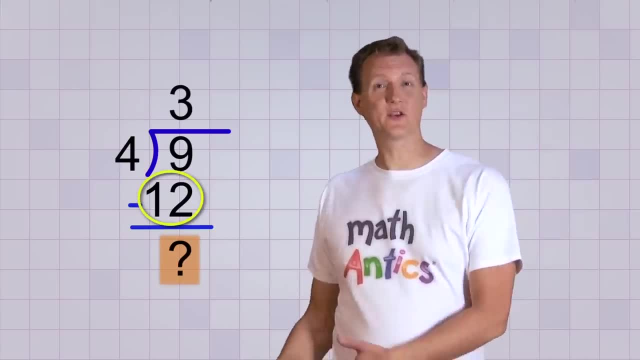 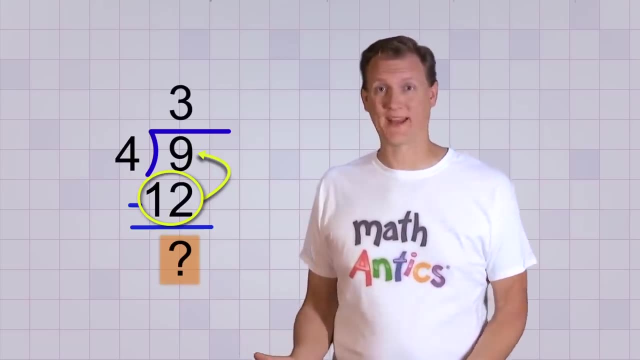 Or can I? This looks like trouble again. The answer to my multiplication is bigger than the number we're dividing up, so I can't subtract it. The remainder would be less than 0.. And I can't have a remainder less than 0. 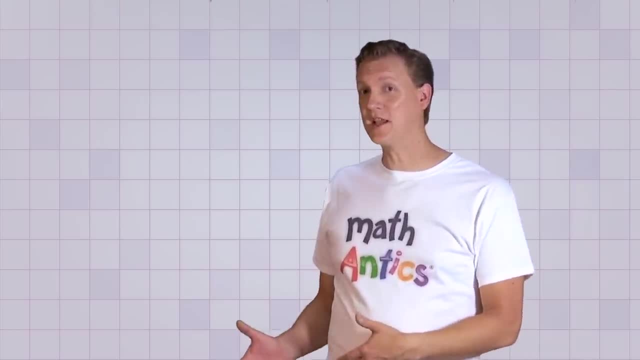 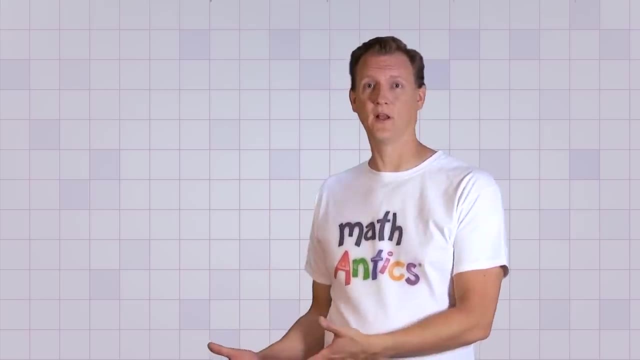 That can't be right. Here's the problem: When you choose an answer that's too big, it's like trying to give too many to each group, And then you run out of things to give before the groups are equal, And if the groups aren't equal, they get all upset. 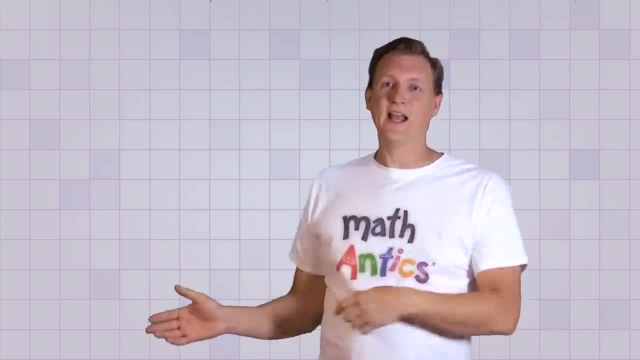 And then, if they get all upset, they start fighting. And if they start fighting, they get upset when the teacher puts them in town, And then they start getting upset, and then they get upset And then the class recess in the hall is over and they don't do that. 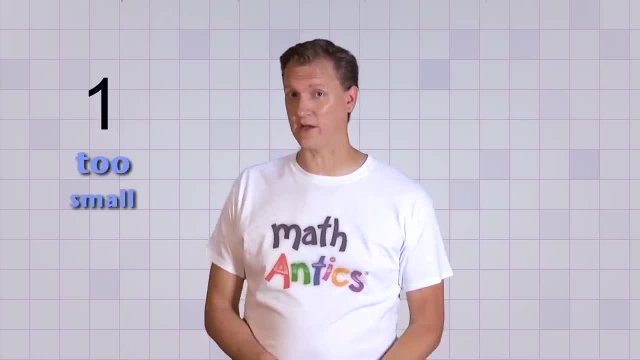 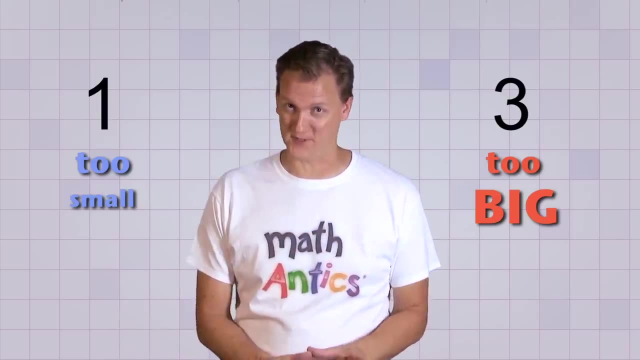 Okay. So 1 was too small. It gave us too big of a remainder, And then they start fighting, And then they start fighting. And 3 is too big. There wouldn't be any remainder at all And the groups wouldn't be equal, which causes big problems. 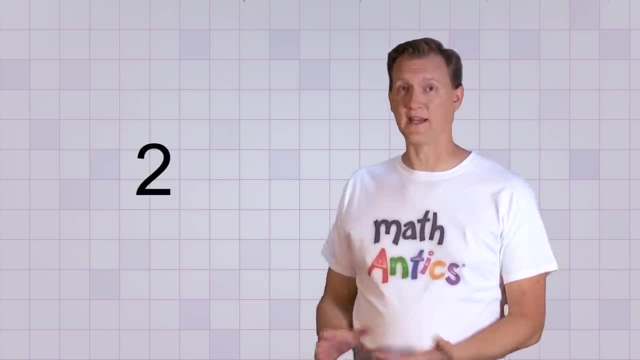 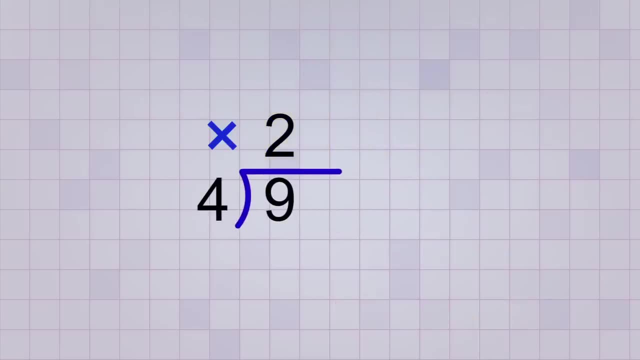 So let's try 2.. If we say that two 4's will make 9, or almost 9,, our problem looks like this: 2 goes in the answer spot, And then we do our multiplication procedure. We multiply that 2 by the 4, and we get 8.. 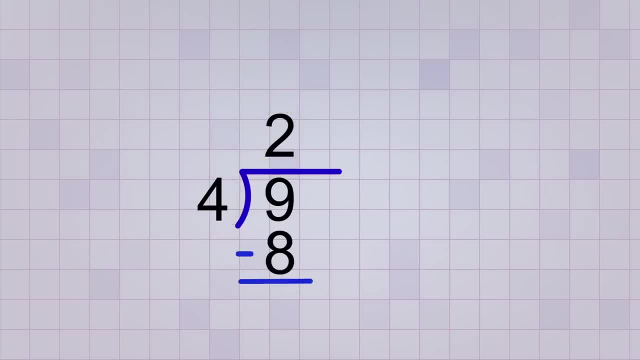 Then we write the 8 below the 9 so we can subtract it and find our remainder: 9 minus 8 equals 1.. So that means our remainder…. So that means our remainder is 1.. Now, that sounds good. It's less than our number of groups. 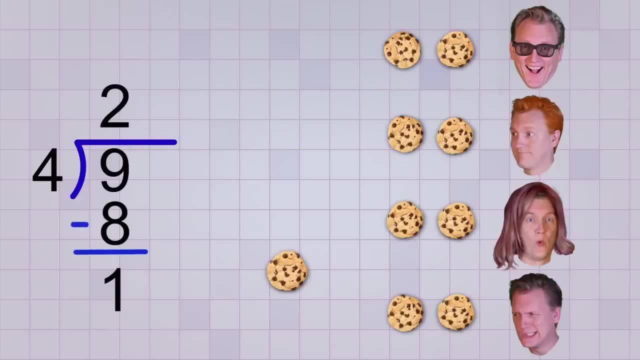 And you can see with our cookie problem that it's exactly right. 9 cookies divided into 4 groups gives 2 cookies to each group, with 1 left over as a remainder which we'll put right up here in our answer with an R for remainder. 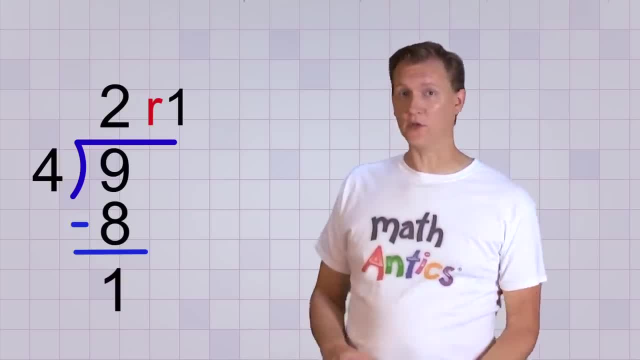 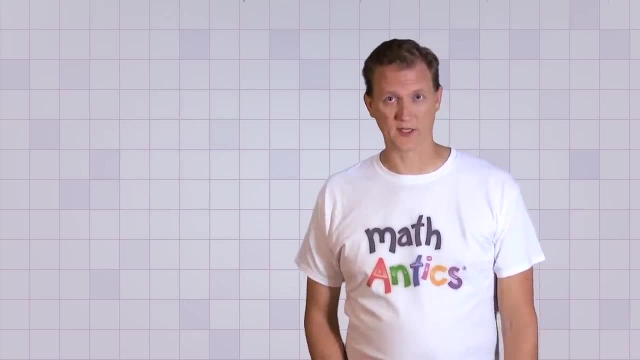 Perfect, And now you can see how you can do division without using pictures or cookies, but just with numbers and a procedure to follow. Let's try a couple more so you really see how it works. Let's try 23 divided by 5.. 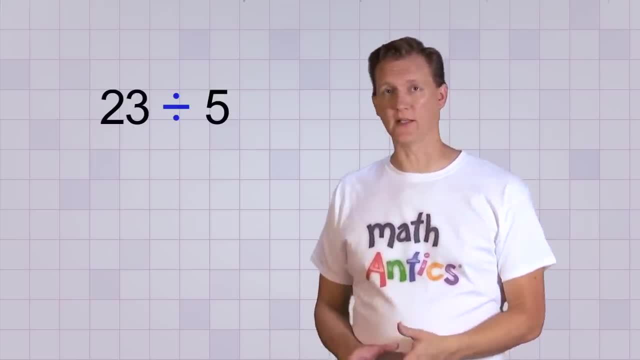 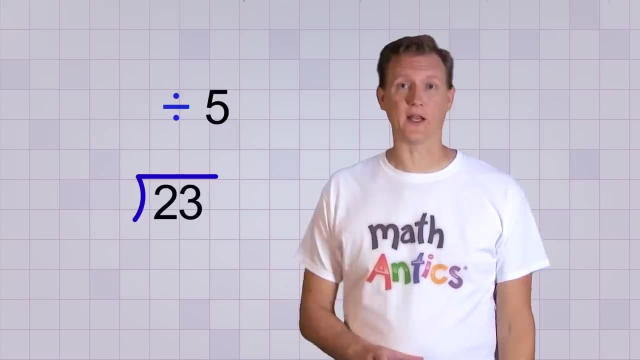 We start, as always, by making sure our problem is written correctly, using our new division symbol. The 23 is what we'll be dividing up. It's our dividend, so we put it under the line. And the 5 is what we're dividing by our divisor, so it goes out front. 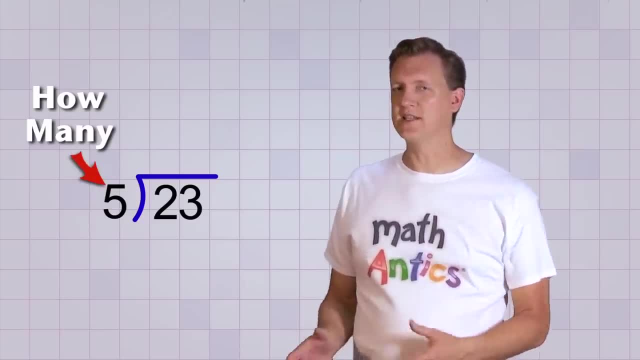 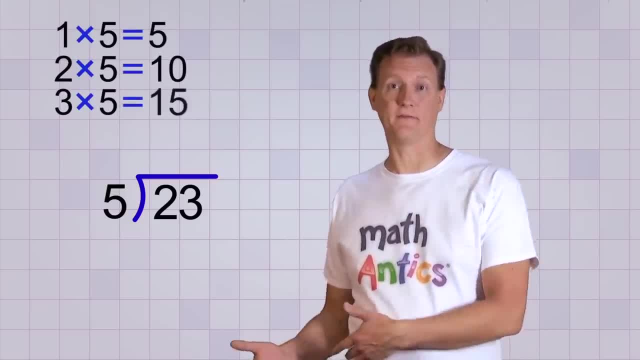 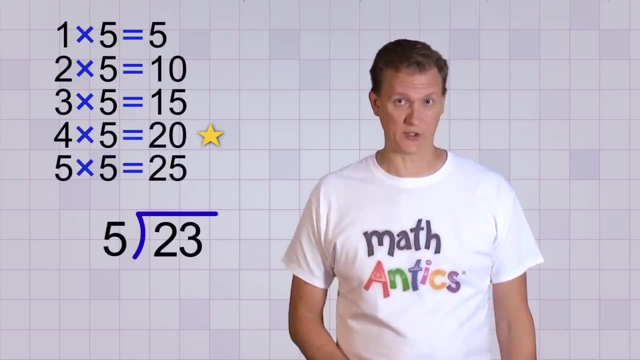 2- 5's is 10.. That's also too small. 3- 5's would be 15.. 4- 5's is 20.. Oh, that sounds promising. Now, 5- 5's is 25, and that would be too much. 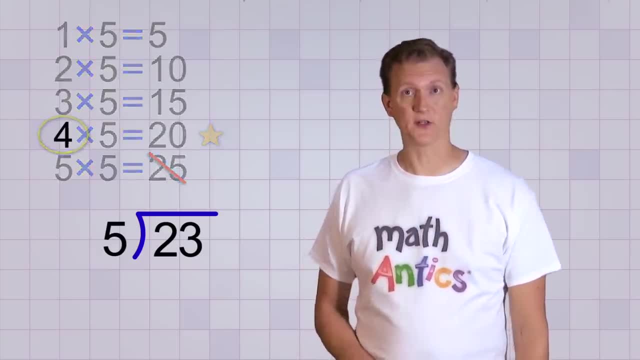 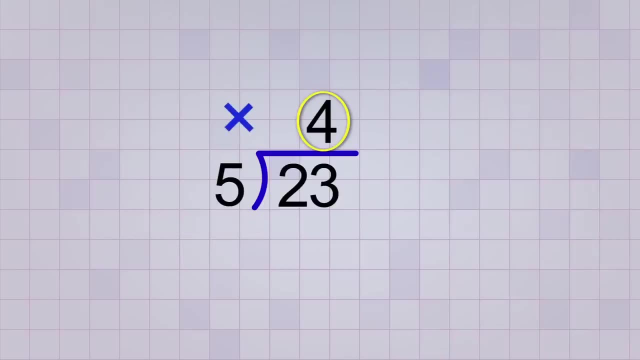 So it sounds like 4 is a really good number to pick for our answer, so let's put that on the answer line. Next we need to do the step where we multiply the answer 4, by the number of groups, 5,. 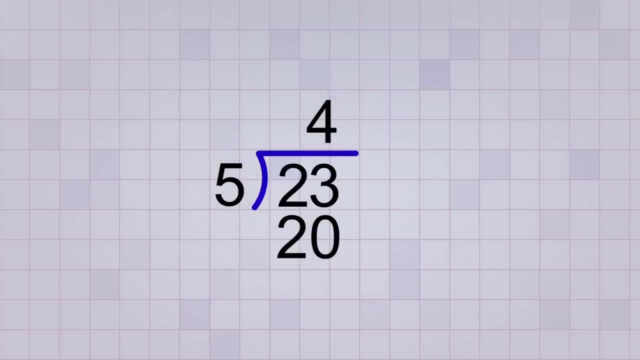 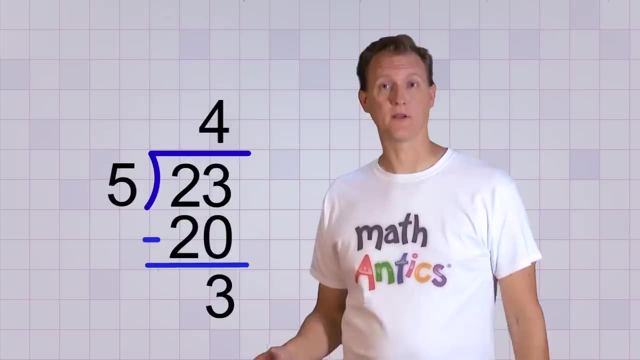 and we get 20, which we'll write below the number we're dividing up 23.. Now we subtract those numbers to see what our remainder is. 23 minus 20 is 3.. Well, that's good. 3 is less than our number of groups, so it's a reasonable remainder. 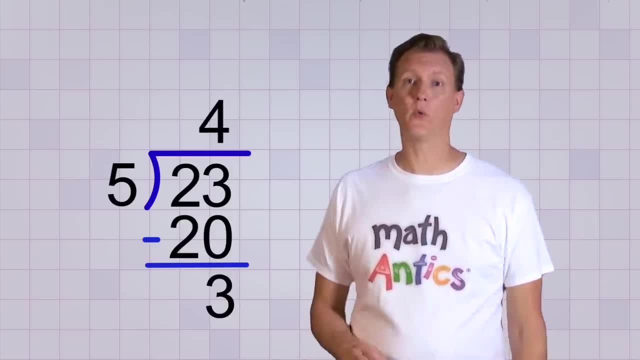 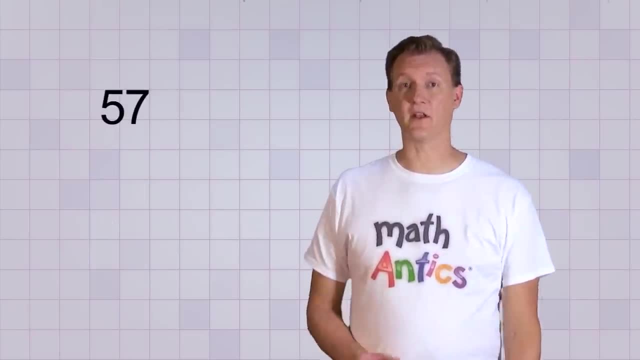 So our answer to 23 divided by 5 is 4 with a remainder of 3.. Let's do one more before you try working some out on your own. okay, Let's do 57 divided by 6.. First we set up our problem and then we ask the question. 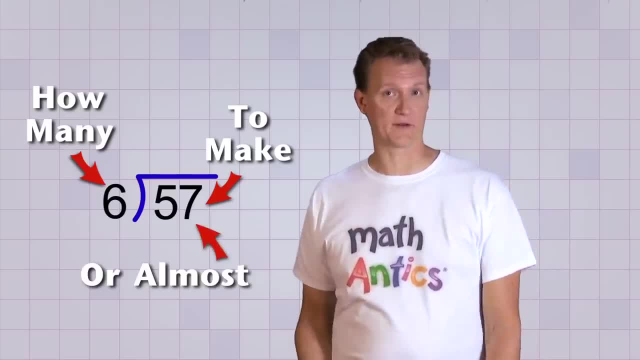 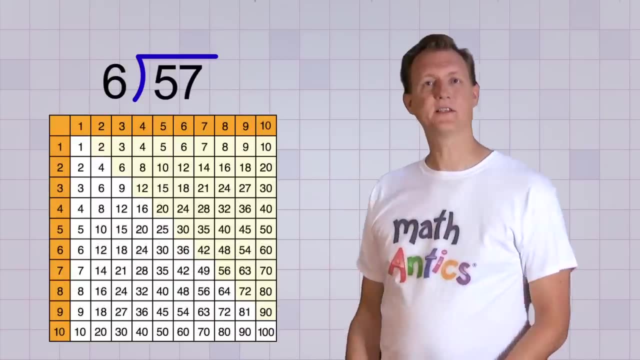 how many 6's do we need to make 57, or almost 57?? Well, this one's a little more tricky, so I think I might use a multiplication table to help me out. The nice thing about a multiplication table is that it shows me all the multiples of a number.